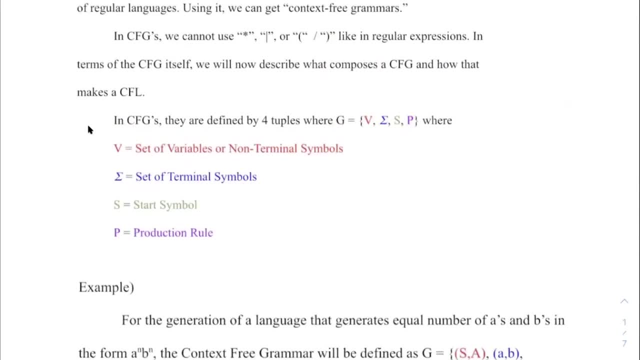 a set of terminal symbols: S equals a start symbol and P equals the production one. So what do all these terms mean? Well, it can be kind of confusing, and I myself, and I assume many of you also, like learning more from the example than the actual definition. 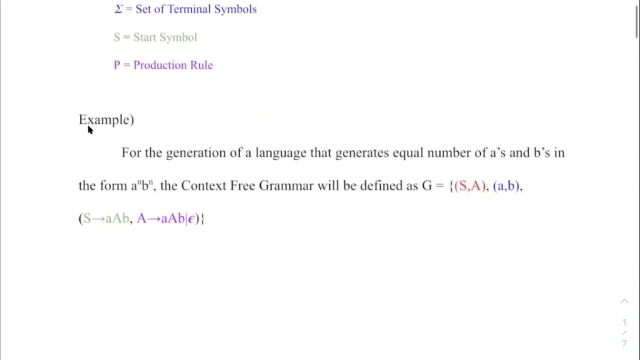 So we'll start off with the example and then I'll explain it a little bit more. So in this example for the generation of a language that generates equal number of A's and B's in the form a, n to the n and v to the n, context-free grammar will be defined. 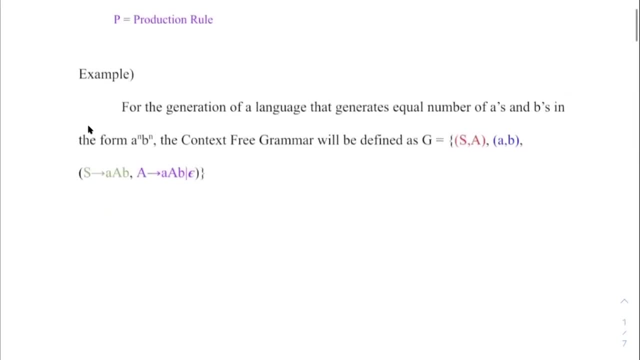 as G equals S A A B, and then S arrow little a big A B, and then A arrow little, a big A B, and then the line is kind of like an or and then epsilon. By the way, if you didn't know, it terminates it or takes it out. 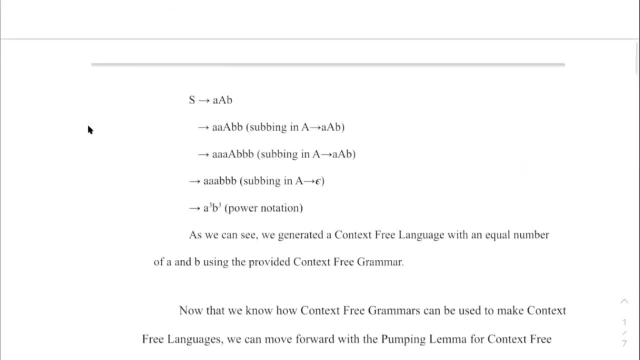 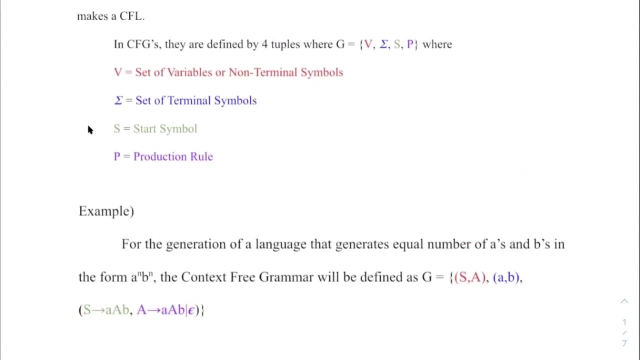 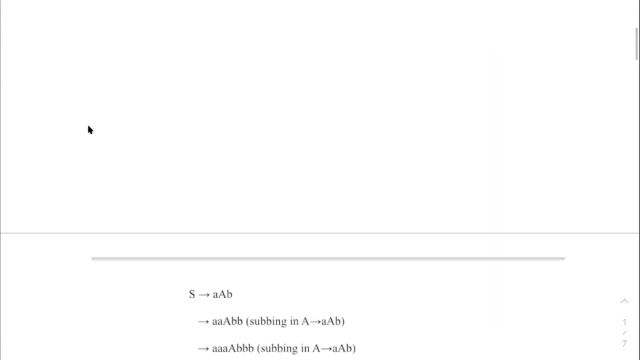 So we'll start here. So we start with S because, as you can see here, which is the start symbol, and the start symbol gives us this right here: the A, A, B. So we sub that in and then so we have this. So what do we do next? We look at the production rule and our rule here. 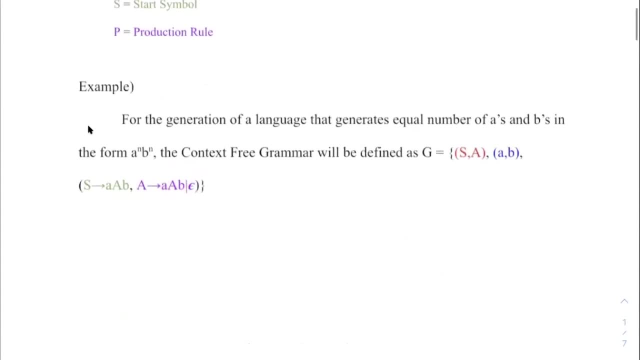 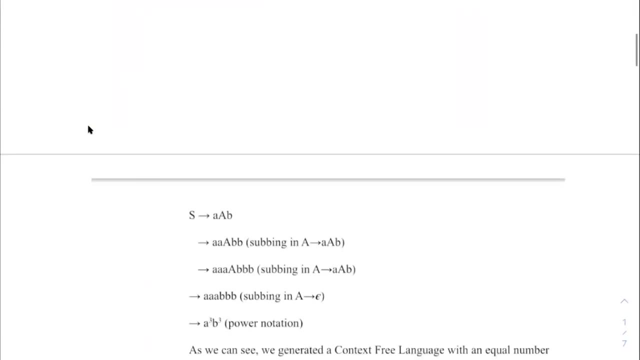 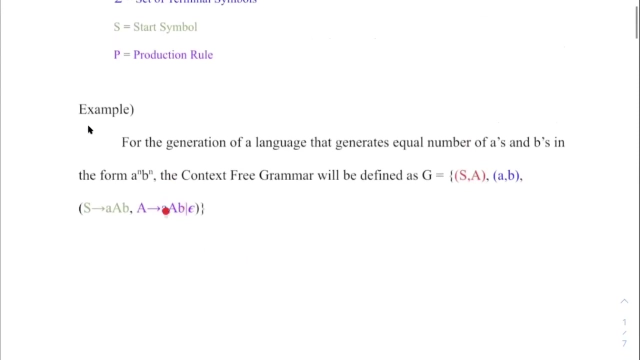 is that it can be used to calculate the number of the number of A's and B's that are present, be the left or the right, and so we take the left, this one, so we submit in, and then we get. this thing is in the middle. here, though, we also have a name, and that's part of our production. 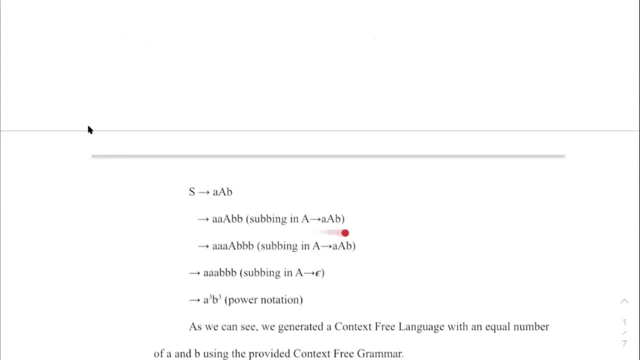 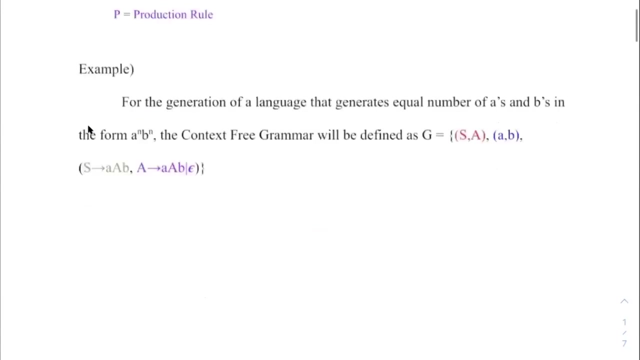 so we're able to do it again right here. so now, instead of this, a a, a, b b, the a, a, a big, a, b, b b. so again we could do it, but instead this time we're going to be doing epsilon. we're able to take it out right here. it's gone now. and the thing is, if we look at what the rules were, 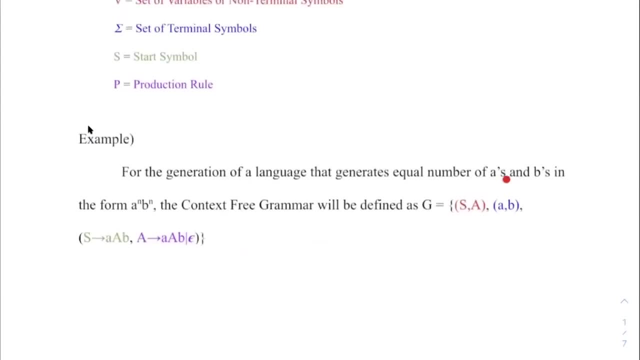 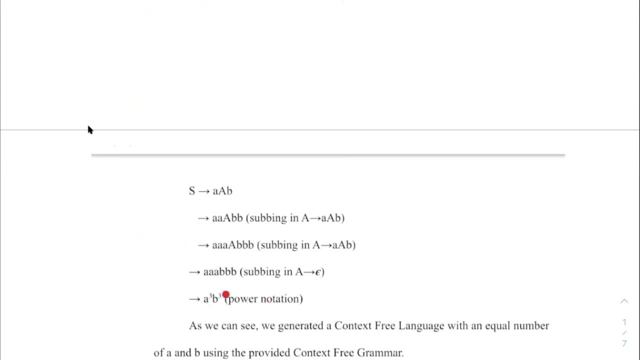 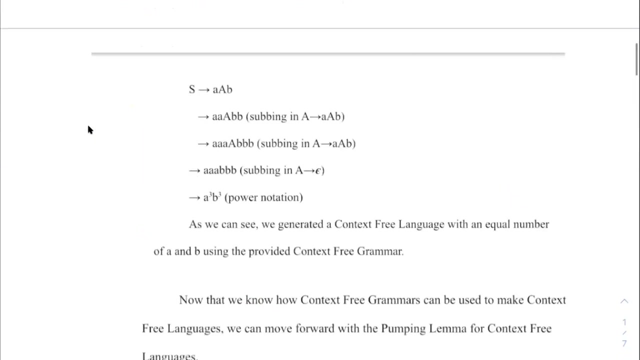 we want the number of a's to be equals the number of b's, so it's a n b n. so when we put it in power notation, we get a cubed and b cubed, in other words a n b n if n equals three. so, as you can see, we generated a context-free language with 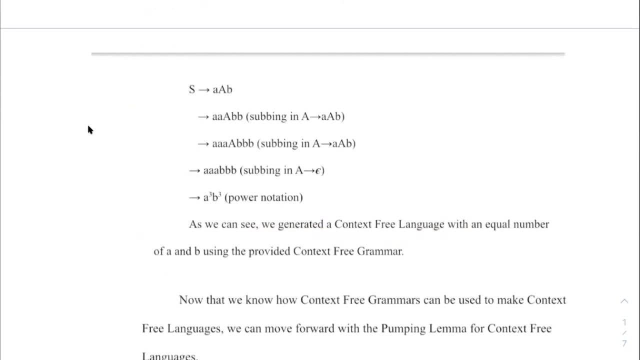 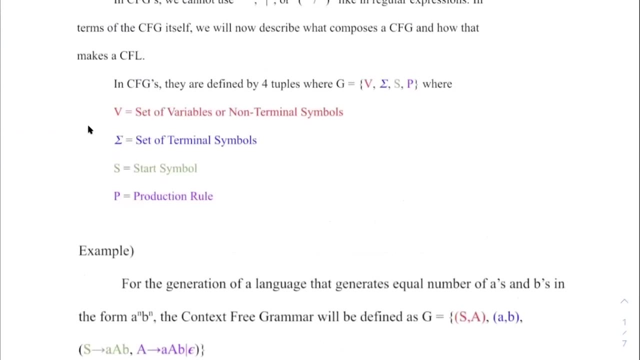 an equal number of a's and b's using the provided context-free grammar and just to backtrack a little bit, because i think you might have a better idea of what start symbol and production rules are. so, as you can see here, blue is a set of terminal symbols. 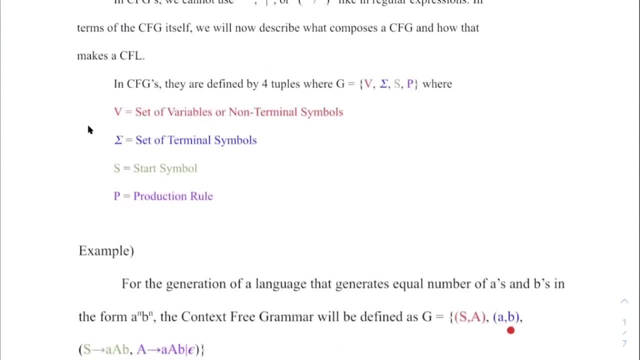 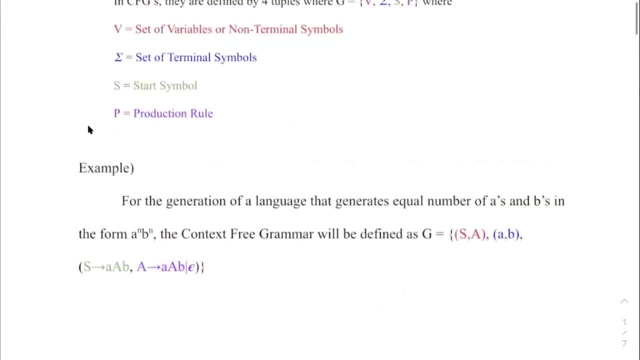 because i color-coded everything and these are the things that we were dealing with, but these are the things that actually like kind of matter. these are the things that are. we're able to sub these things into. so it'll be like this way, or if you all draw it out this way. so for the a's, 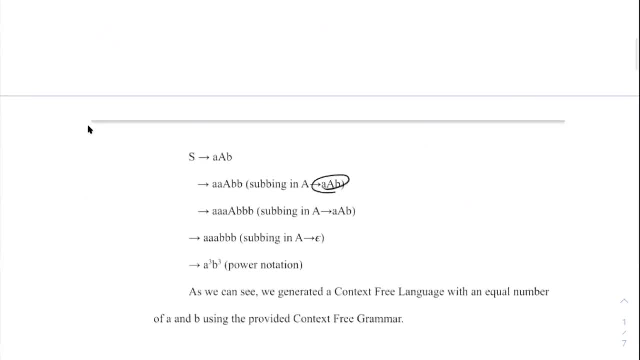 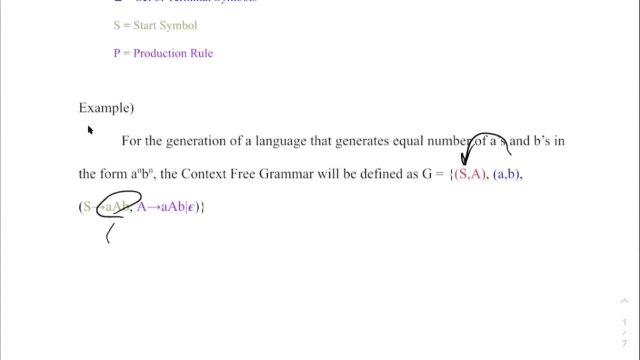 we were able to sub it in with this right here and for the s's. that's what gave us our story, and so the ending is straight forward, and we know that these are starting state here. i guess it is important to point out that the starting state here is equal to what we're. 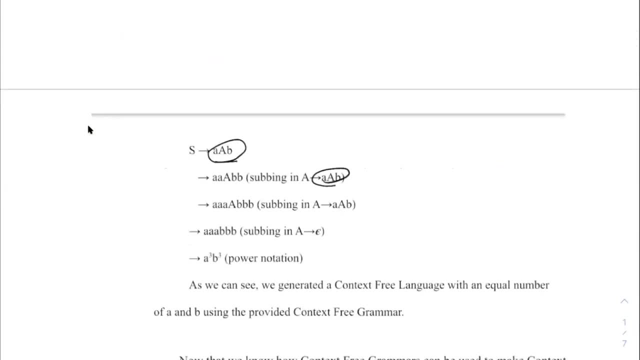 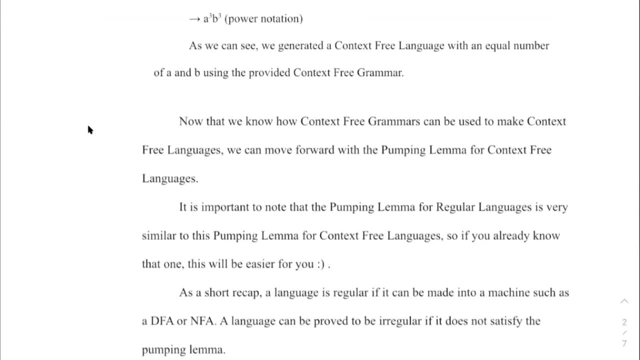 subbing in, which is why it's pretty straightforward for an example, but that's why they're starting examples, to be honest, um, okay, let's move on. now that we know how context-free grammars can be used to make context-free languages, can you move forward with the same problem? 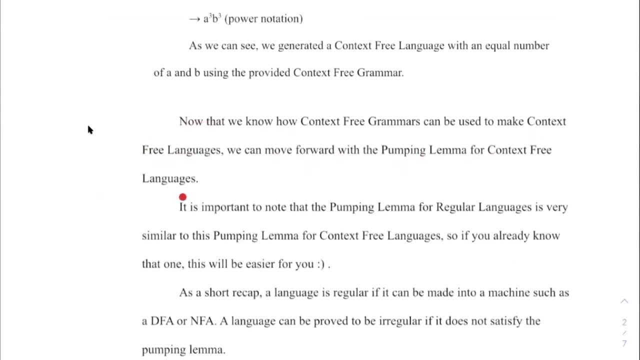 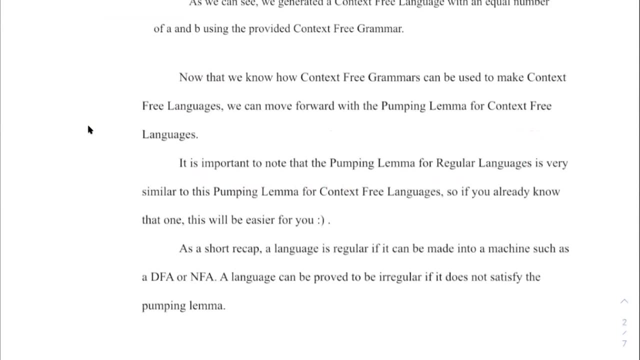 or with the same concept, or even please use the different problem options to come up with, move forward, the pumping lemma for context-free languages. So it is important to note that the pumping lemma for regular languages, what we've talked about previously in this class- is very 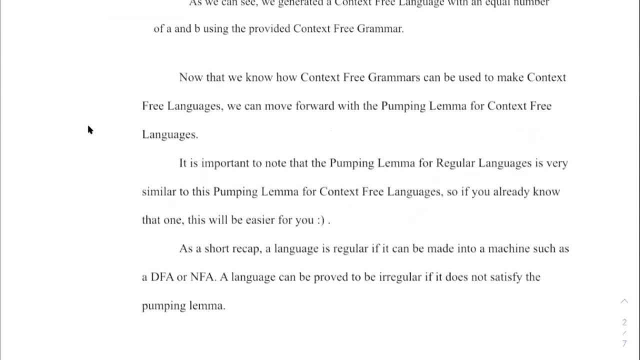 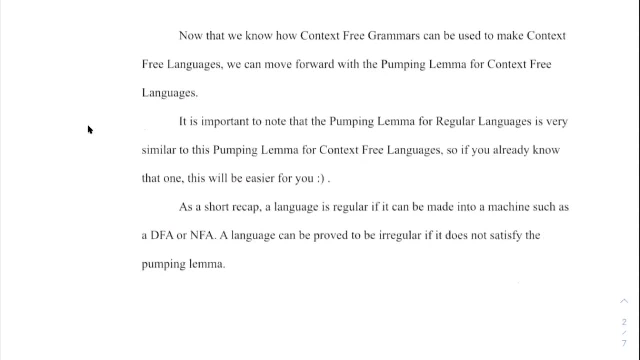 similar to this pumping lemma for context-free languages, So if you already know that one, this will be easier for you, which is honestly pretty nice because they're related somewhat. As a short recap, language is regular if it can be made into a machine such as a DFA or NFA. 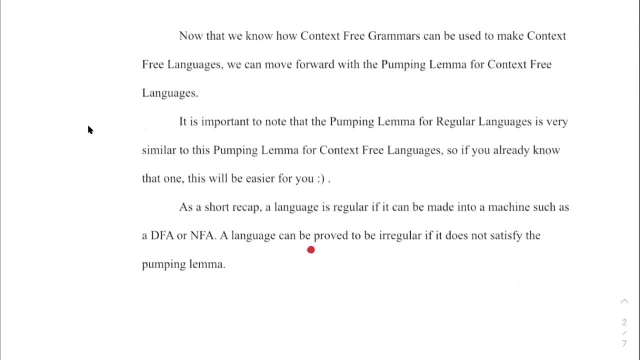 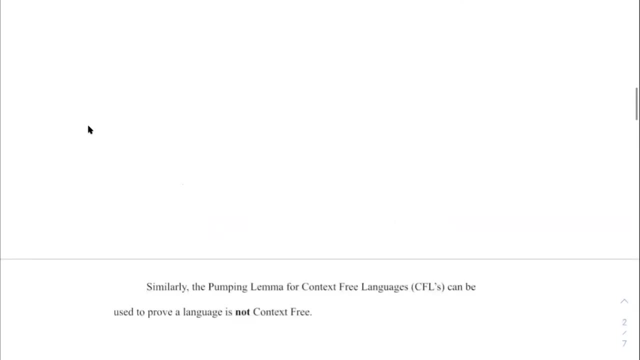 However, in this case, a language can be proved to be irregular if it does not satisfy the pumping lemma, Like that. This is where, in this case, Similarly, the pumping lemma for context-free languages can be used to prove a language if it is not context-free Before what we talked about. 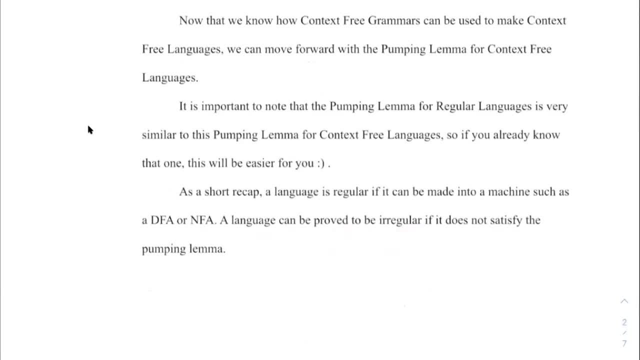 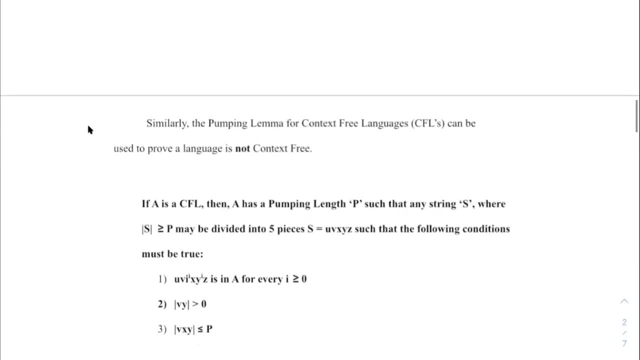 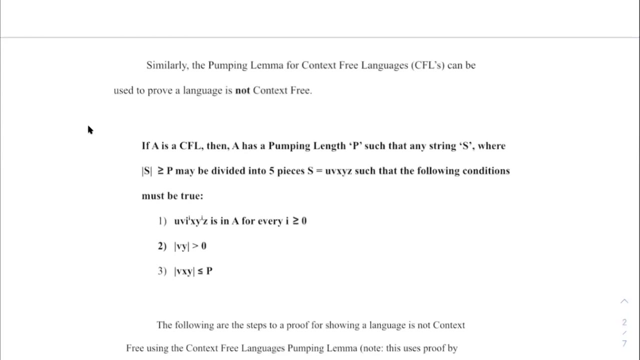 is proving a language is irregular by not having satisfied the pumping lemma. In this case, if it does not satisfy the pumping lemma, it will be because it's not context-free. So these are kind of just the rules overall of the pumping lemma for context-free languages. So 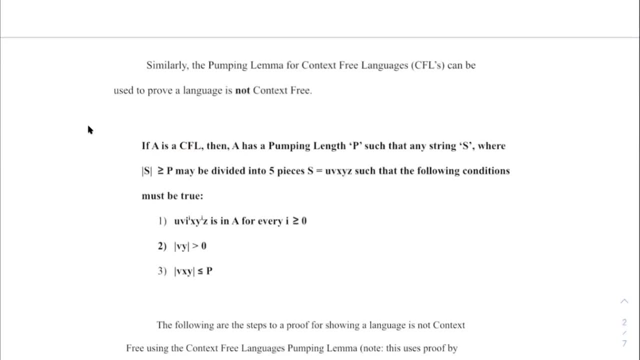 if A is a context-free language, then A has a pumping length, P, such that any string S, where the length of S is greater or equal to the pumping length, may be divided into five pieces. So if S is equal to the string, then it'll be divided into pieces U, B, X, Y and Z. 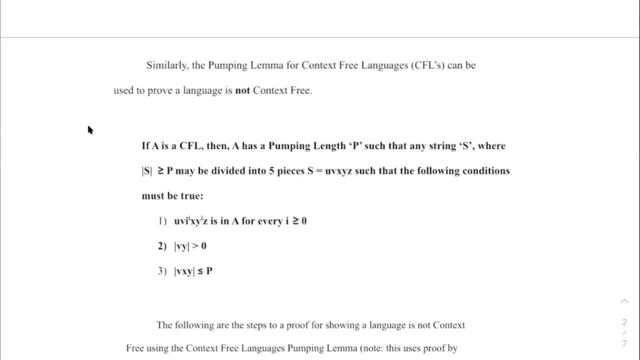 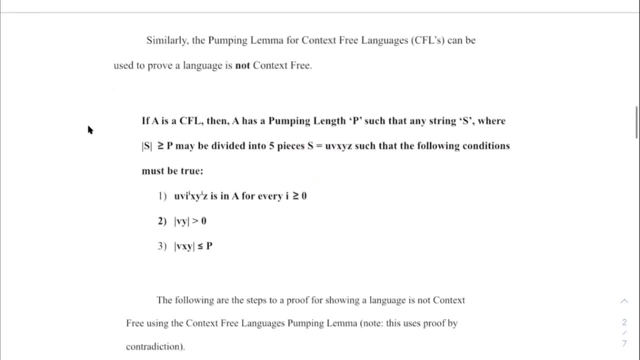 And it's important to note, just because the pieces of the string does not make them a string. they're just parts of the overall string And such that the following conditions must be true: These pieces must follow these conditions. So U and then V. I to the power of I. 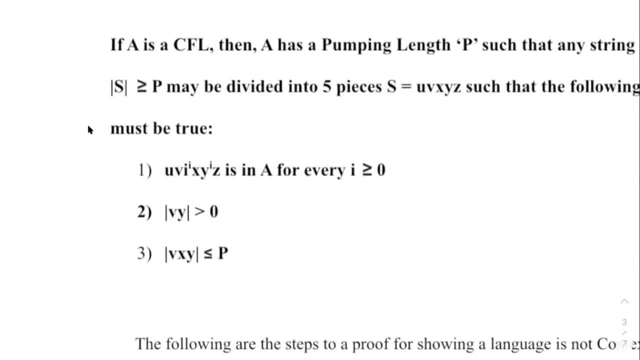 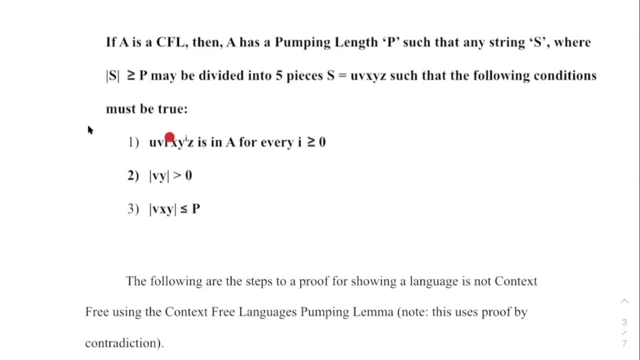 X, Y to the power of I and Z is an A for every I greater than or equal to zero. And this is just pretty much saying that for these powers of I which are greater than or equal to 0, they just have to match these powers. 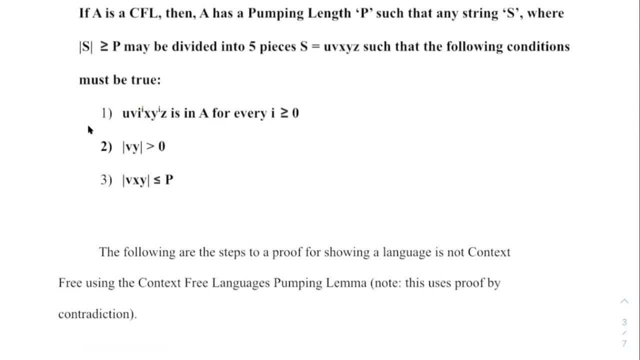 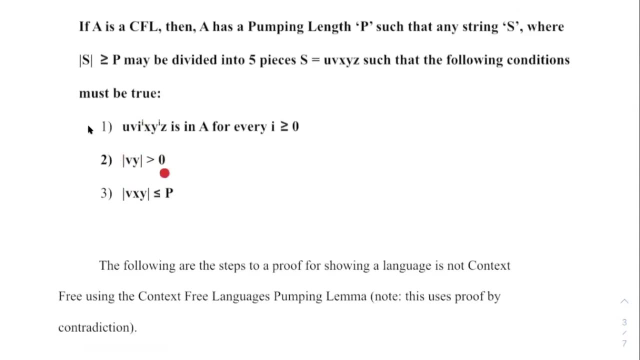 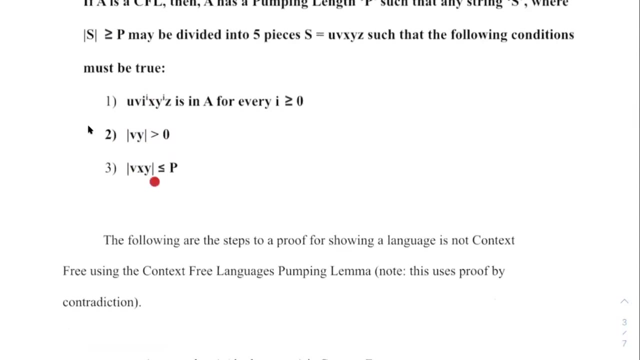 And yeah, so specifically the I and the Y. Here it's saying that for the parts V and Y, the length of these two must be greater than zero. And then, finally, final condition, is that the length of V, X and Y is less than or equal to P pumping length. Those are the three conditions, And so, in order to pass the 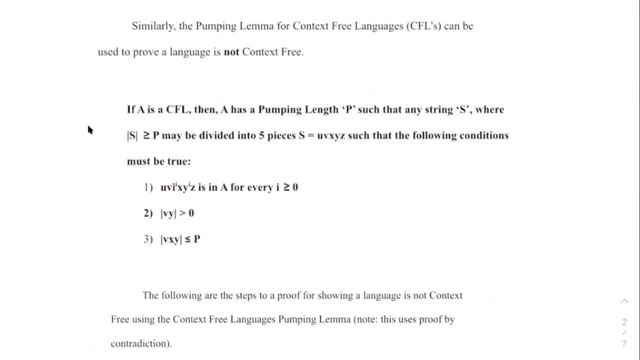 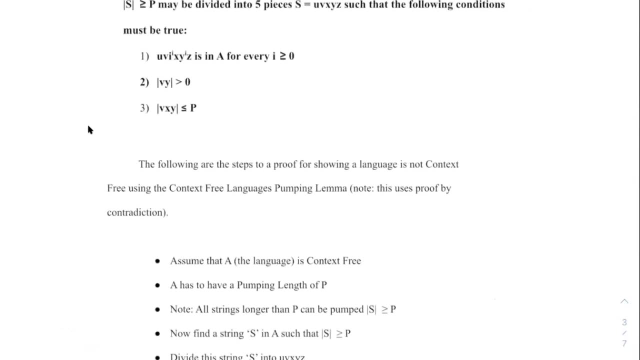 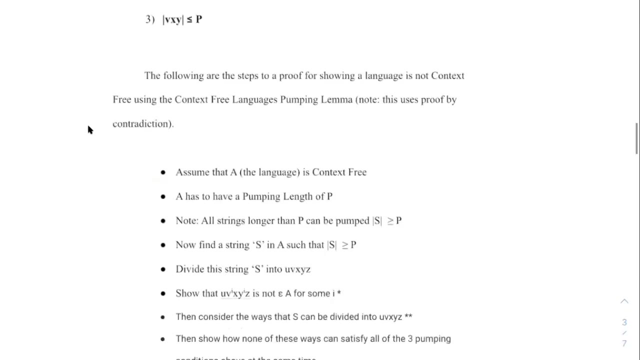 pumping lemma. all three of these must hold or be true. So the following are the steps to a proof for showing a language is not context-free using the context-free language of pumping lemma. And note, this does use proof by contradiction. So oh, of course, let's start off with the proof. 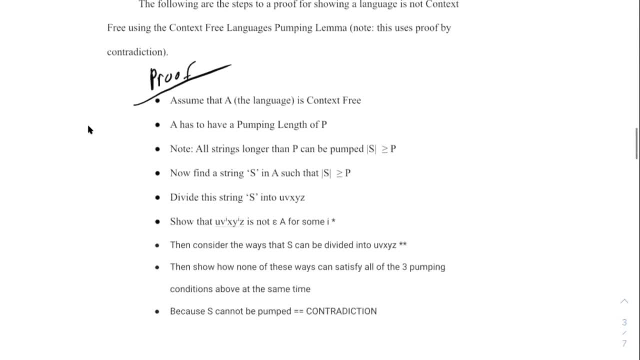 That's always important. Assume that A, the language, is context-free, Let's use the pointer again right here. So we're saying A to the language. A has to have a pumping length of P. Note: all strings longer than P can be pumped. 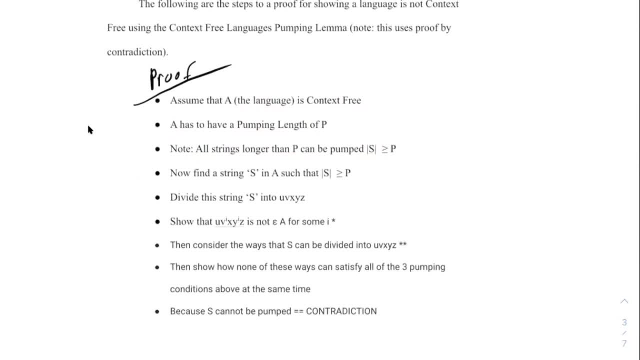 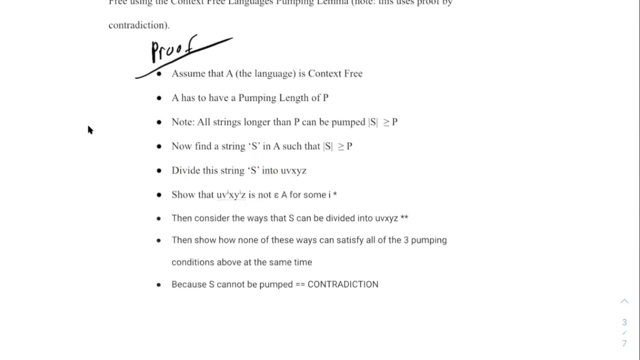 By the way, the absolute value symbols denoted here represent length, So the length of any string longer than P can be pumped. Now find a string S in A such that the length of S is greater than or equal to P pumping. So dividing this string S into these five parts, which are U, V, X, Y and Z. So we divide it. 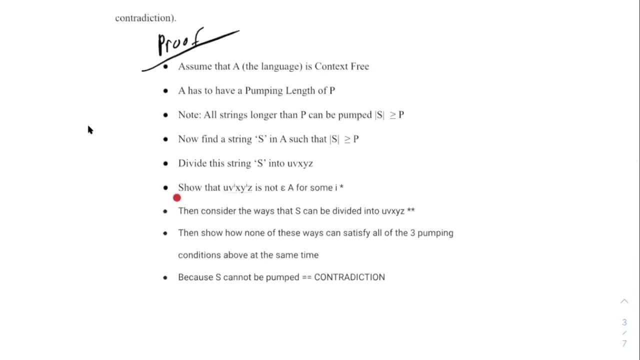 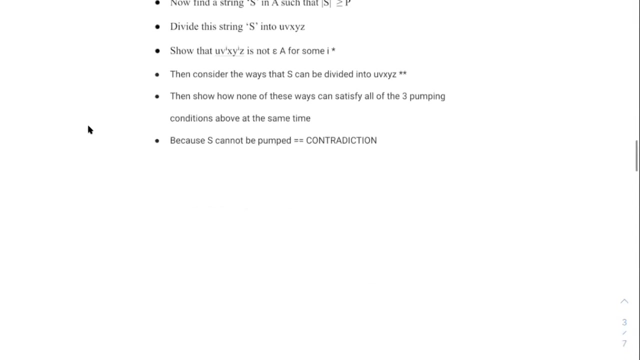 And then we will have show that U, V to the I, X to the Y, I, sorry, and Z is not well. epsilon A for some I And then I. in my notes myself I define it as: 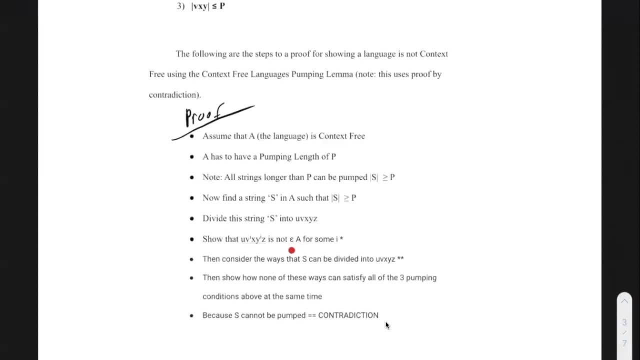 here in U, V to the I, X, Y to the I, Z is not within A. So then we consider the ways that S can be divided into U, V, X, Y and Z, And this then separates the proof into cases. So then show how none of these ways 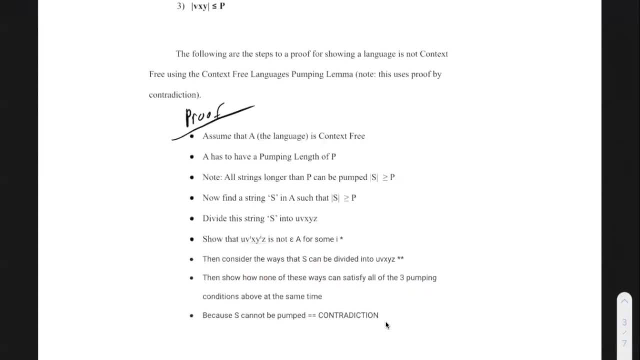 or these cases can satisfy all of the three pumping conditions above at the same time. So this: if this doesn't work, then we don't even need to check the proof. So we need to check these two. But if this works, then we have to check this one And then 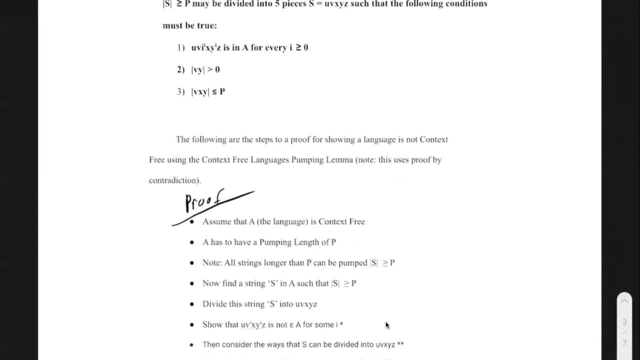 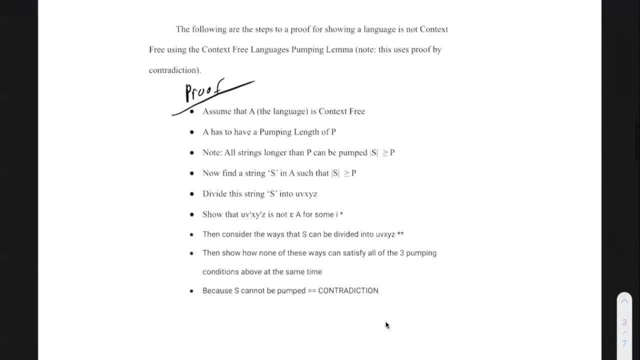 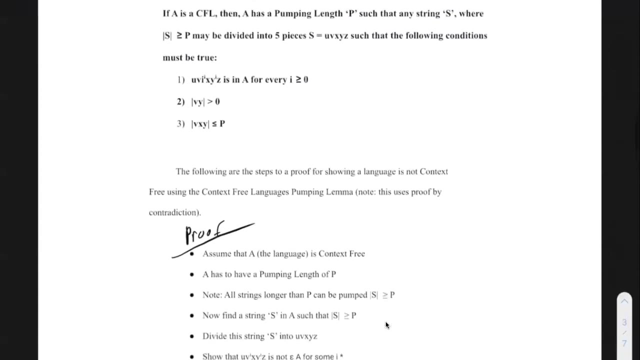 if this one works as well, then we have to check this one. All three of them need to be true, or it has a pumping moment for a case, And then usually, if for some reason it cannot be pumped from one of these conditions, then there's a contradiction and it is not a context-free. 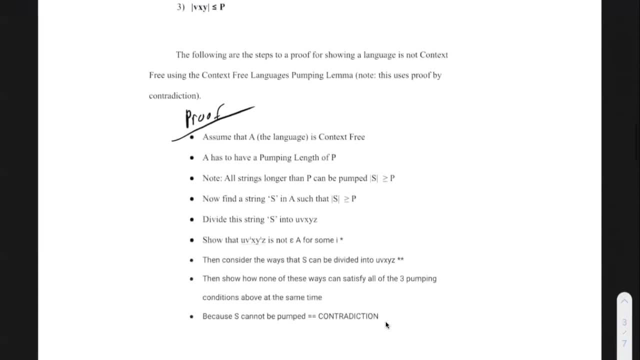 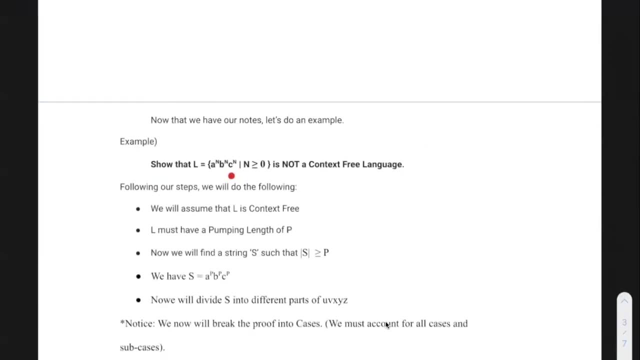 language. So let's move on to an example. why don't we Show that L equals A to the N, B to the N and C to the N, and N is greater than or equal to zero? This is how. this is not a context-free language. So, following our steps, we will do the following: 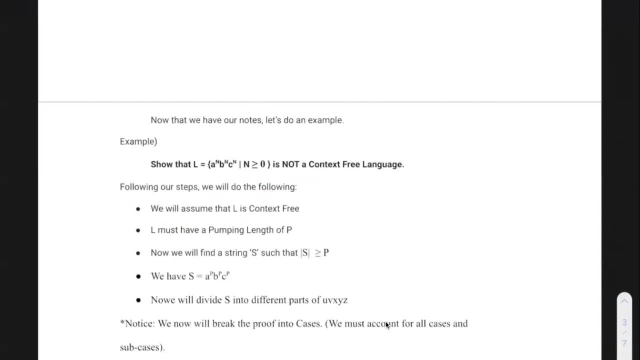 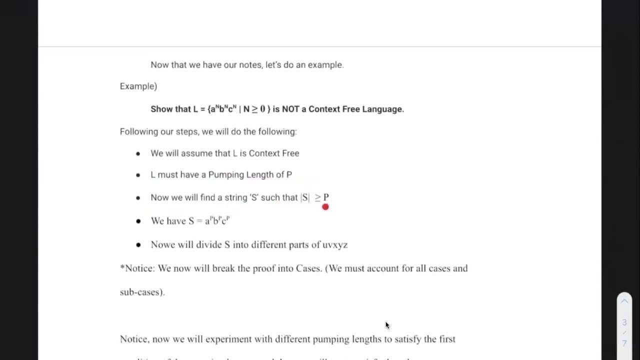 We will assume that L is context-free and L must have a pumping length of B. We're just following our steps here from what we went over previously. Now we will find a string S, such that the length of S is greater than or equal to P. 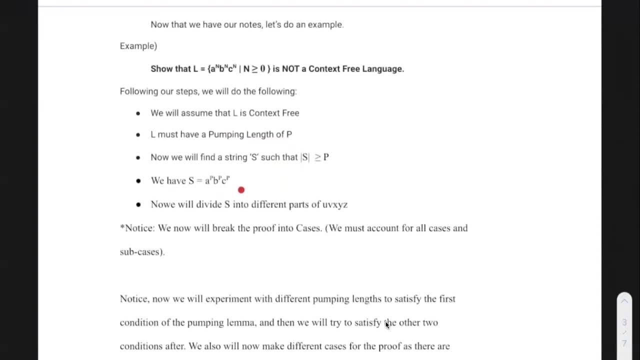 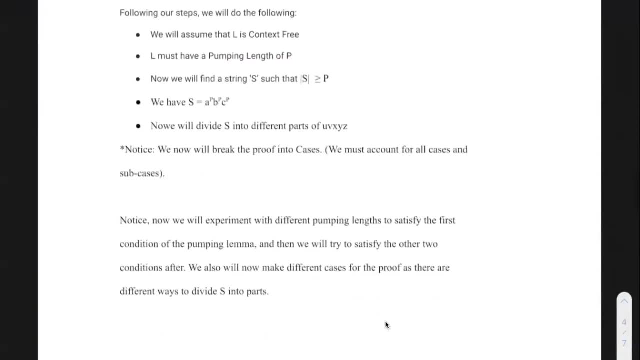 So we have S equals, and then A to P, B to P and C to P, where P is representing the pumping length stated here. Now we will divide S in the different parts of U, V, X, Y and Z. 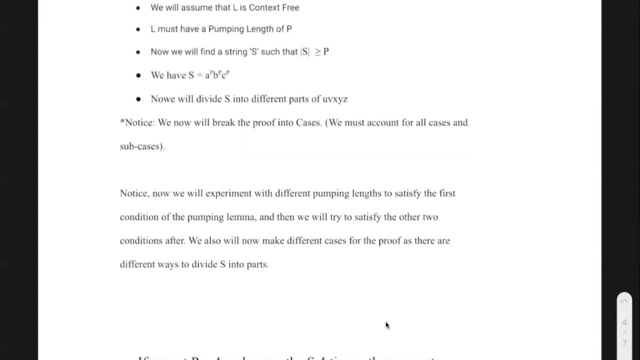 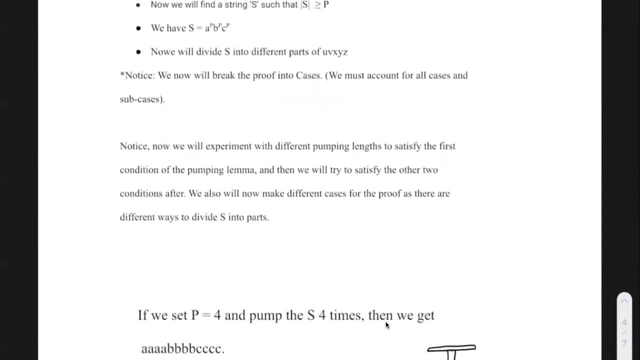 So it is important to note. we will now break the proof in the cases. We will stick out for all cases and subcases. So we will experiment different pumping lengths, aside for the first condition of the pumping length and then tomatoes, by the other two conditions after. 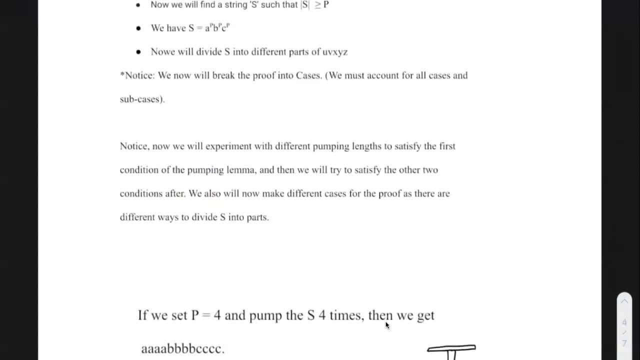 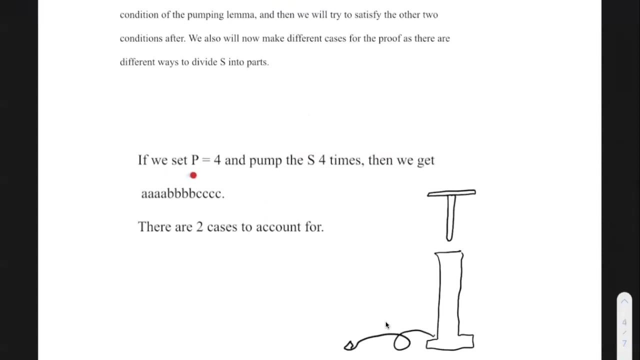 Sorry, it's not as much pumping lengths as much as it is combinations, and we will see in a sec. We will also now have make different cases for the proof, as there are different ways to divide S into proofs. So in this case, um, we set P equal to 4. as we stay here, We will experiment different. 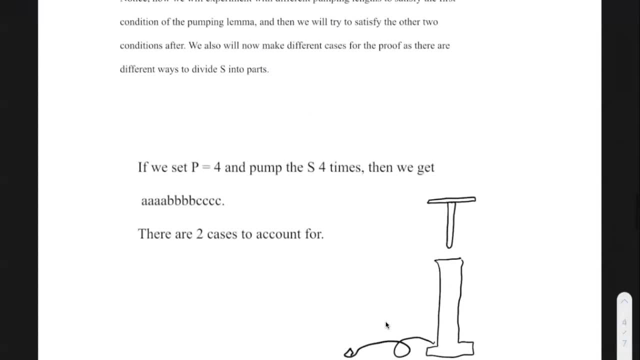 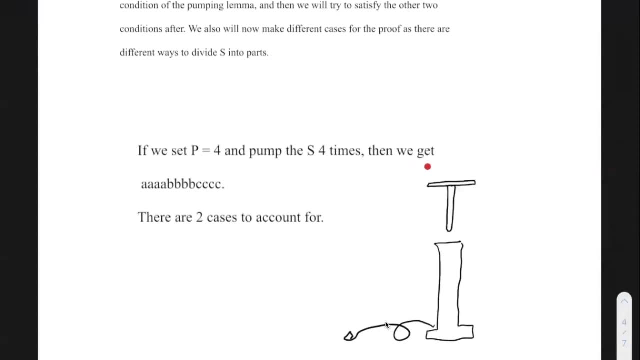 pumping links. but not just that, Don't forget. we're also going to be experimenting with the different options. We set p equal to 4 and pump s four times the string. So kind of do like this: This is just for fun, but if it's a pumping link of 4, we're going to do 1,, 2,, 3,, 4.. And what does? 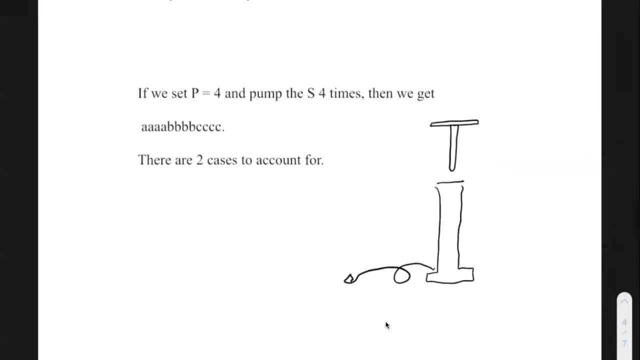 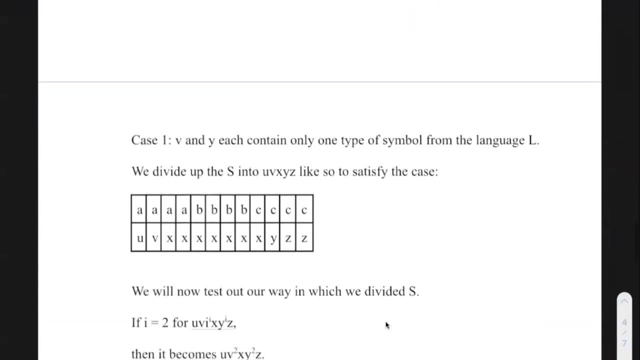 that mean for the string. exactly. That's fun, Because our string looks like this and the n is affecting the pumping link, or in this case p, it'll be duplicating each one. So we have the original a, but then we also have the next one, next one and next one, So four pumps. 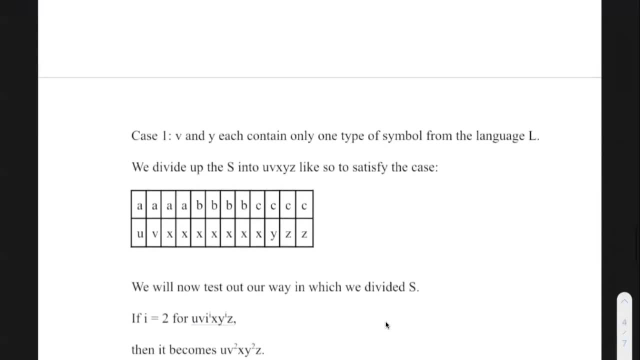 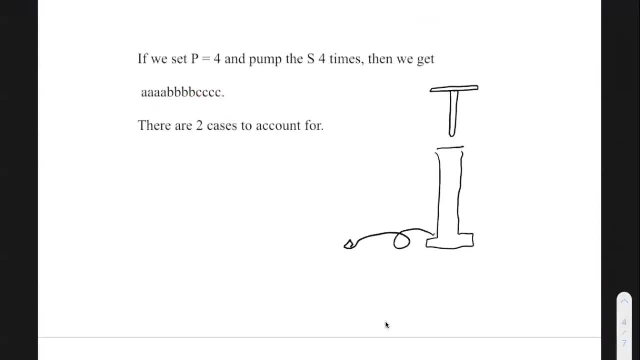 means four a's, four b's, four c's, And this gives us two cases that we need to account for. So I already figured out the cases for you guys, but actually the cases that we need to account for are the ones that we're going to be using. So we're going to use 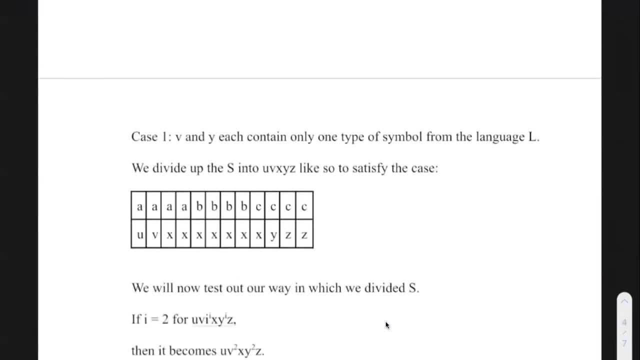 some of the hardest parts of the pumping lemma. So if you do want to get better at pumping lemma, you do have to figure out your cases. So case one, the v and the y each contain only one type of symbol for the language L. These are the things that we're breaking up into. So parts v and y each. 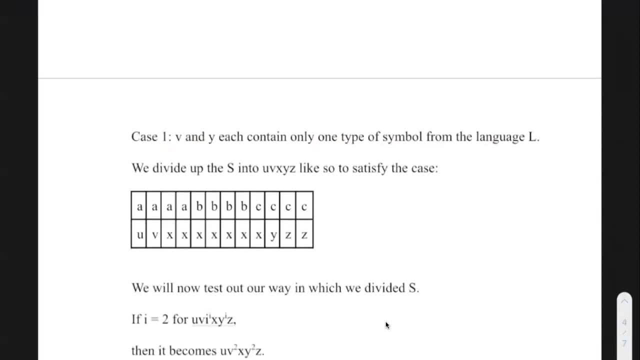 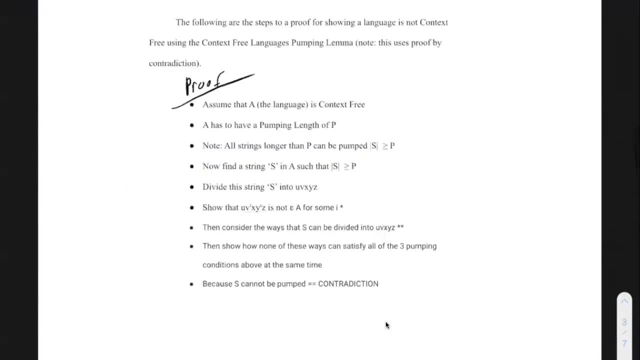 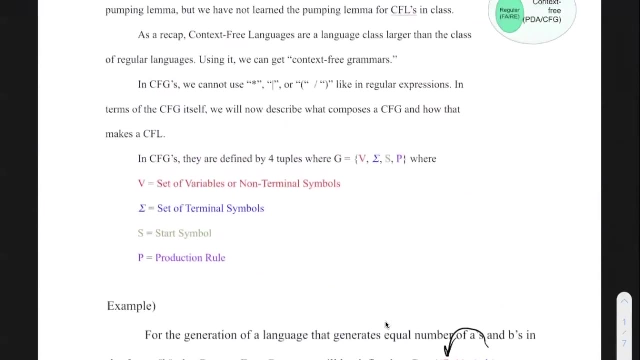 contain only one type of symbol By these terminals. going back to our definitions, at the very beginning, we have a set of symbols for the language L, So we're going to use the terminal symbols. I'm sorry, I almost mixed things up, So that is what we are talking about. 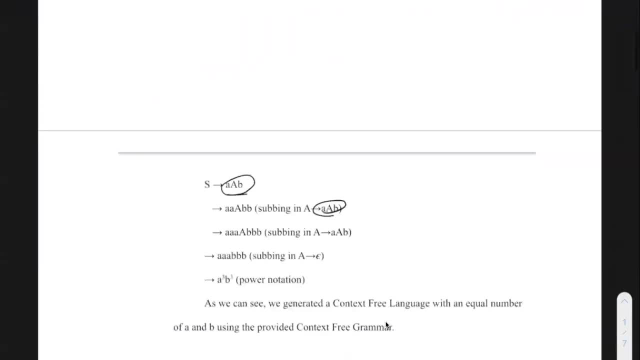 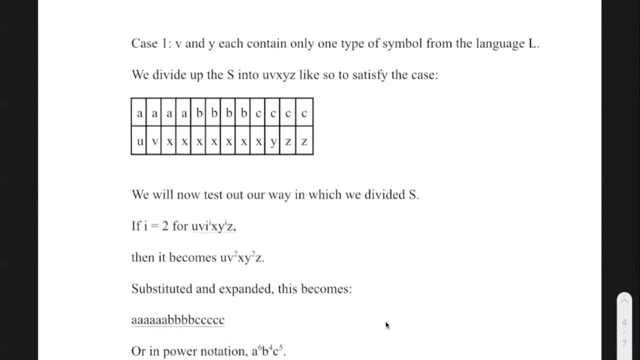 We can only contain one of those, So I already did the work for us here, but you just are assigning it. So for the u, we only get an a, one a P, we only get an a X. we get multiple though, So we get. 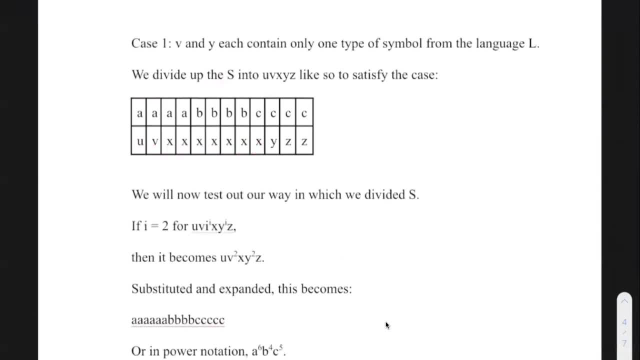 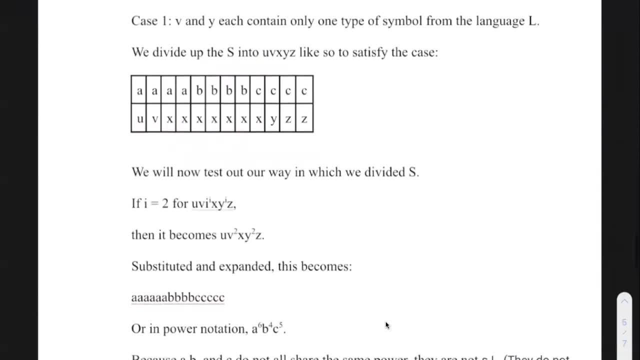 a, a, b, b, b, b, b and then c. So x actually has three different types. Y has one type and it's only a, c, And c has two c's but only one type. And, as you can see here, 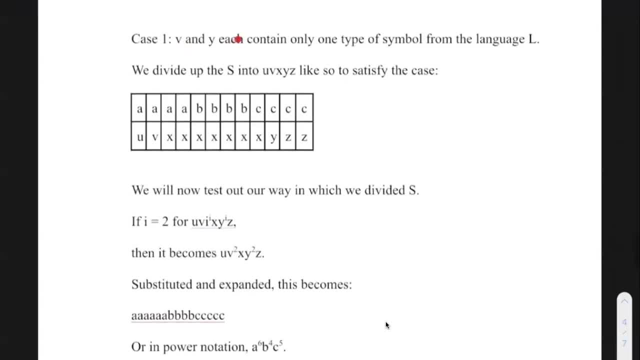 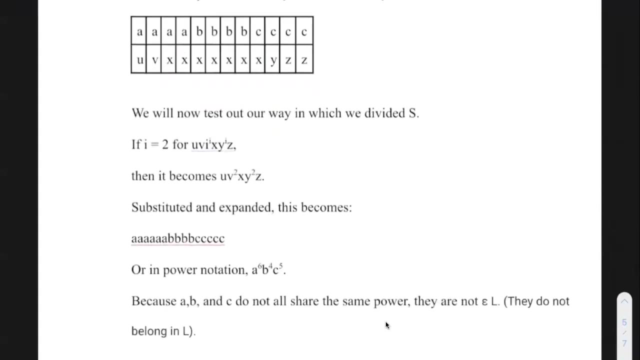 v and y each only contain one type of symbol, One one, one a, one c. So now we can actually test it. Let's see if it satisfies the conditions And if i equals two for u v, i to the i. 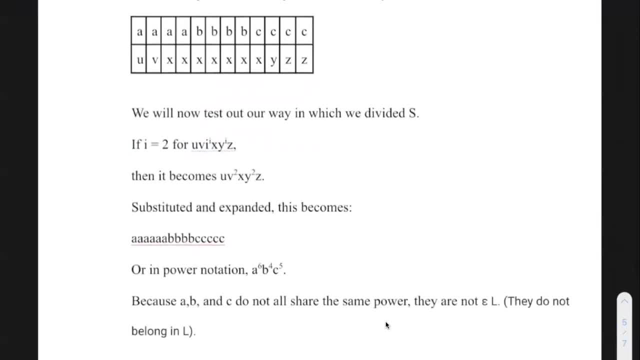 and x, y to the i, z, then it becomes u- v, squared x, y to z And substituted in and expanded. using this chart here, or just the way that we divide to split it up, we get a, a, a, a, b, b, b, b. 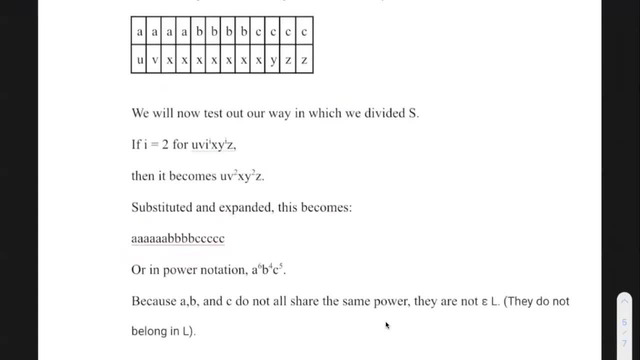 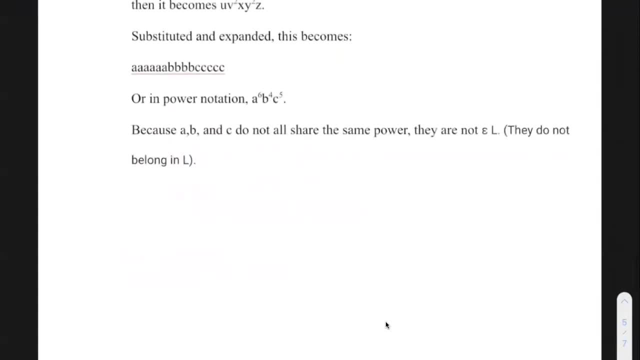 and c, c, c, c, c For our entire notation, because that's a lot more organized: a to the sixth, b to the fourth and c to the fifth. But here's a problem: These should all have the same powers. So because 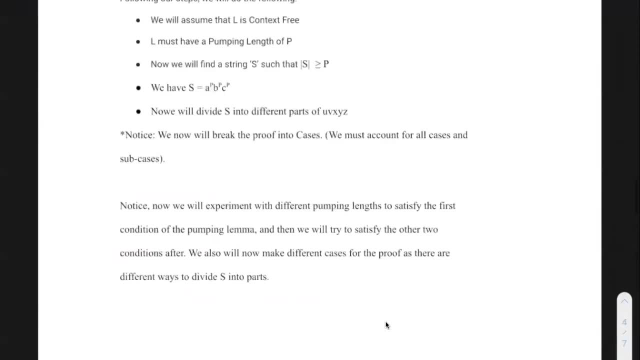 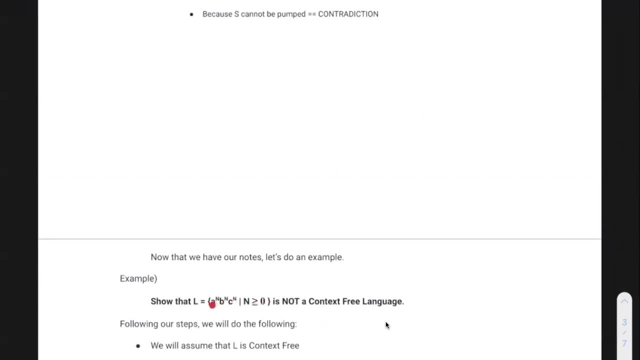 by the way, that's what it said in the example right here. they're all to the same power of n, So they should be having the same powers, but they don't. Kind of weird, right We have, because a, b and c do not all share the same power. they are not. epsilon l. 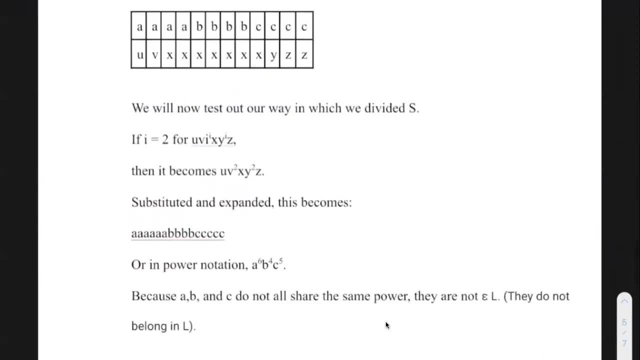 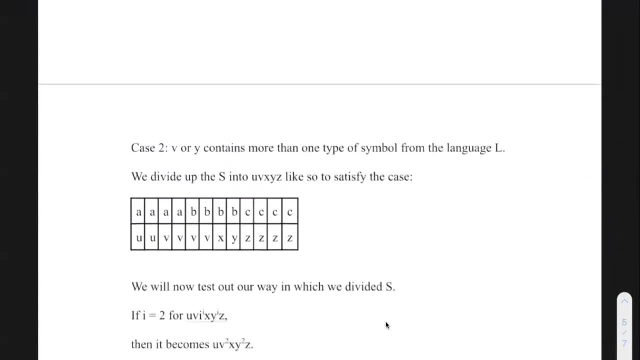 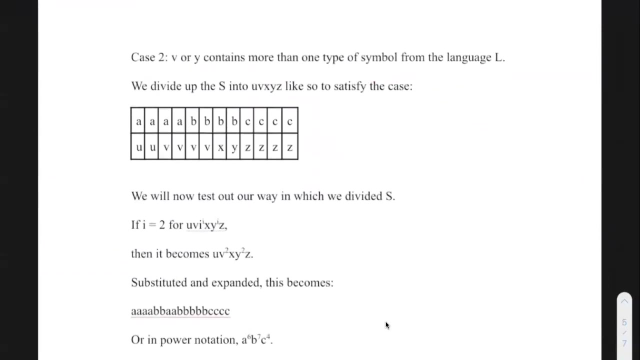 They do not belong in the language Interesting. So what about other cases, right? So our final case, case two, the v or y contains more than one type of symbol from the language l. So, using this principle, this time we're going to make sure that they contain more. 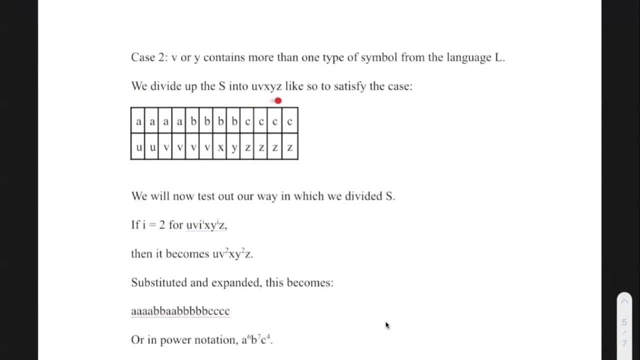 than one type of symbol or so it doesn't even both of them from the language l, And again, I did divide it up just for the sake of time. but here we go. So a, a and the u, so u has one type, b has multiple types, as it wants here. 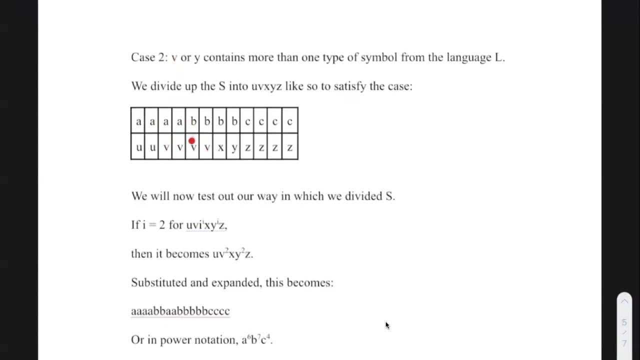 So a, b, so two types here. this time x has one type and y has one type. So in this case y has one type and then it's actually these that have two types, And the z's have one type, the c's 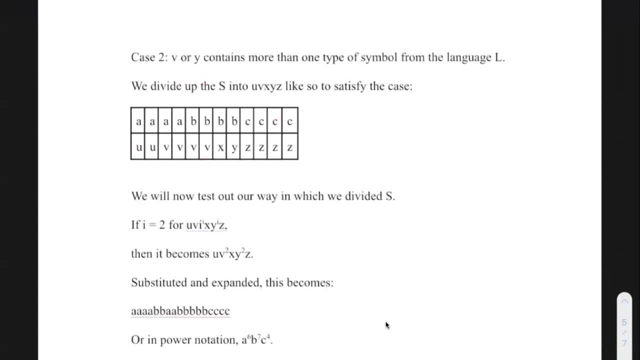 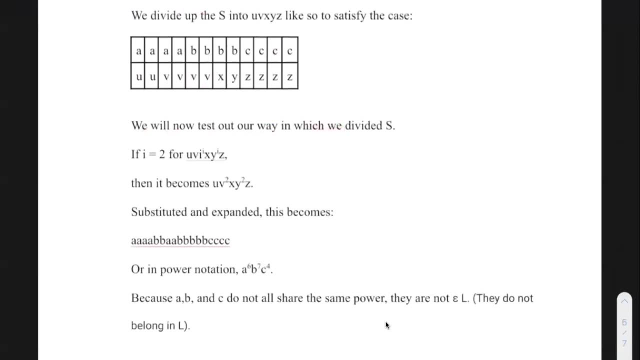 So we are satisfying this and we split up correctly. We'll now test out our way in which we divided s right here. So if i equals two for this pattern, or the way that we split it up, and it becomes u, v squared x, y squared z, 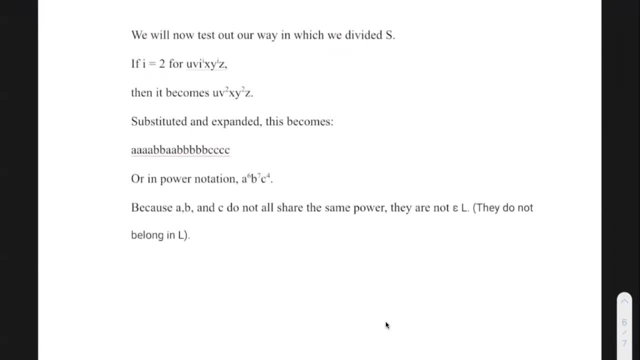 When we sub in these values here into this and expand it, but based on the powers, this becomes this, That becomes this. So we have a a, a, a, b, b, a, a, b, b, b, b, b, c, c, c, c. 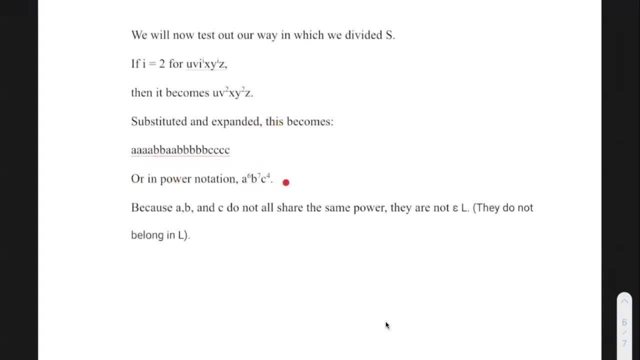 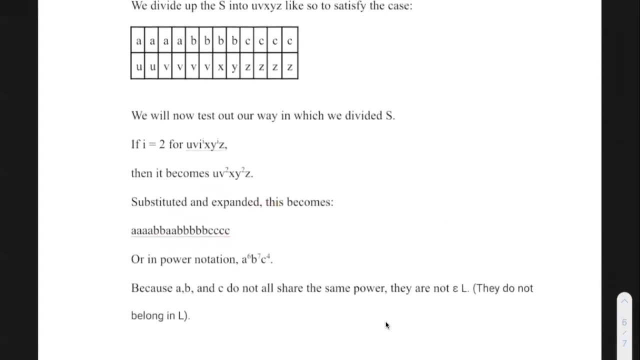 Or in power notation: a to the sixth, b to the seventh, c to the fourth, And, just like our previous example, these both do not share all the same power, which is what we need in this problem. So therefore, they are not in l, They do not belong in l. 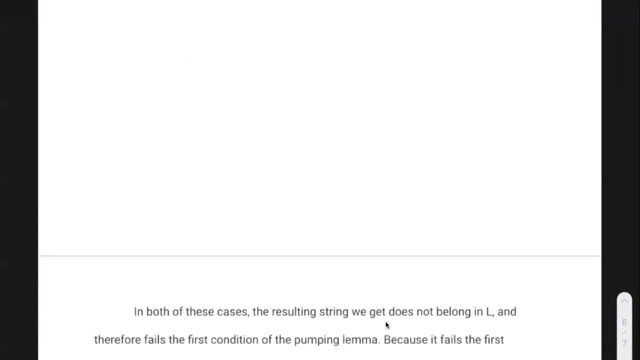 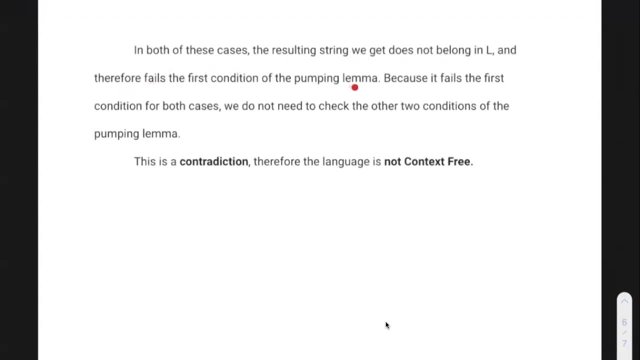 So what does this mean exactly? In both of these cases, the resulting string we get does not belong in l The language and therefore fails the first condition of the pumping lemma. Because it fails the first condition for both cases, we do not need to check the other two. 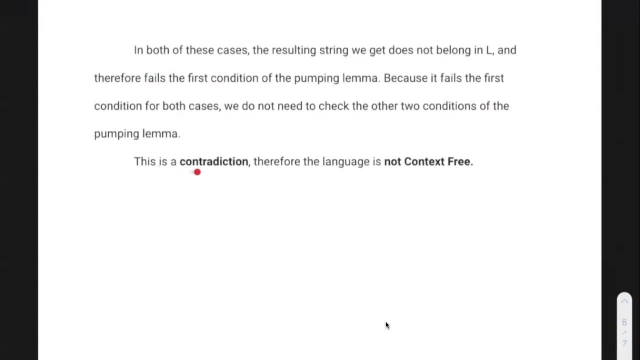 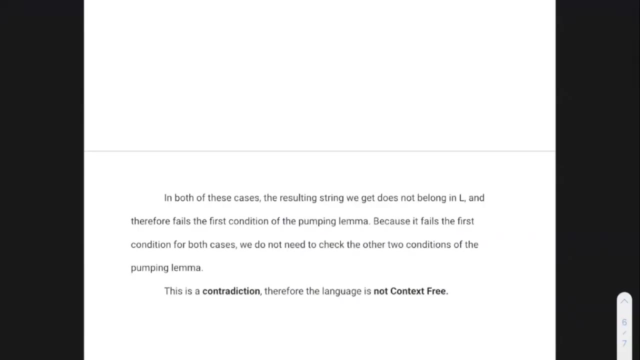 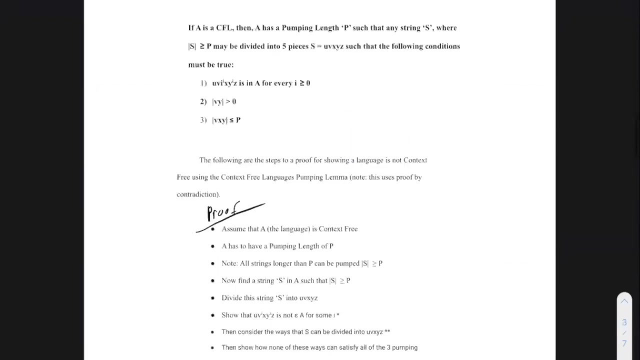 munitions of the pumping lemma. This is a contradiction. Therefore, the language is not context-free. Cool, Thank you. All right. so now that we did everything, I'll just be going over it really quick because we have some more time. Let's go to this part. 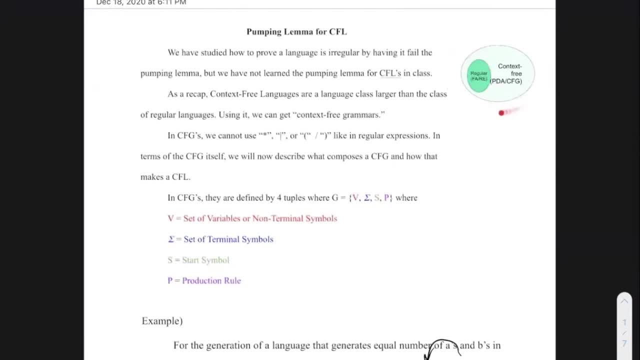 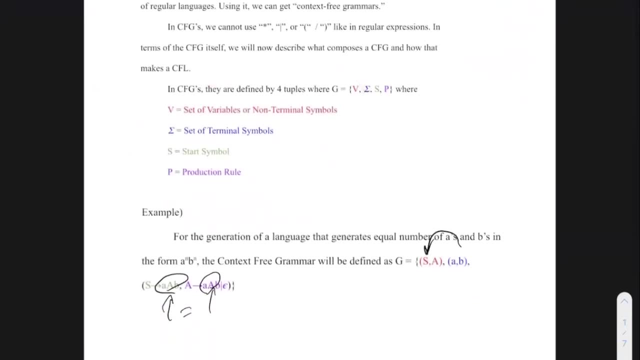 We talked about how regular languages are within these cfgs, and cfgs slash cfls are what we were talking about today. These cfls are composed of four parts, and what you mainly have to worry about is what we're starting with in the production. These are the things we're dealing with. 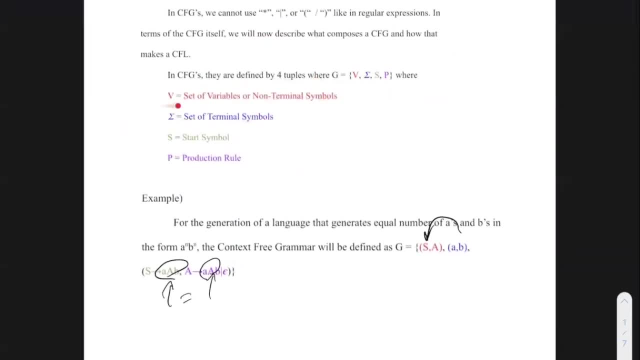 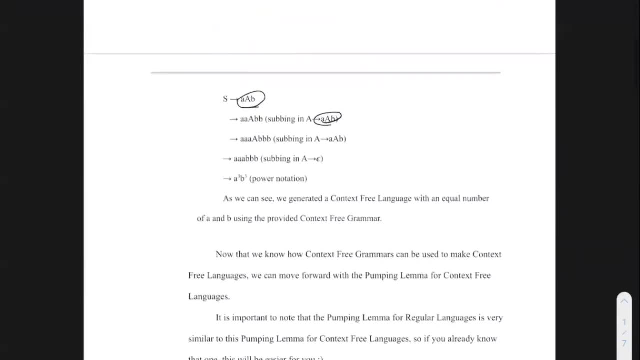 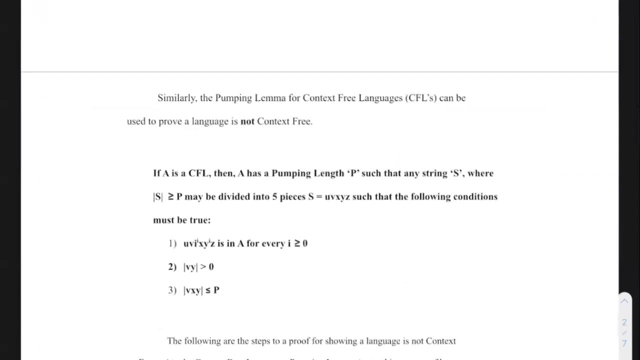 the blue and these are the things that we're kind of using to represent these blue, and then we sub stuff in And we did the example and just kind of talked about it and we actually learned the rules. So we have the pumping length feet and just the general thing is. 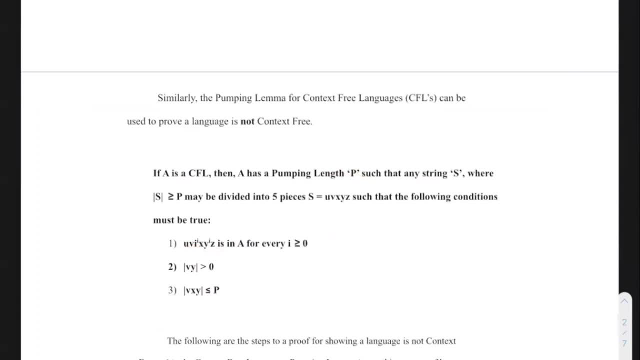 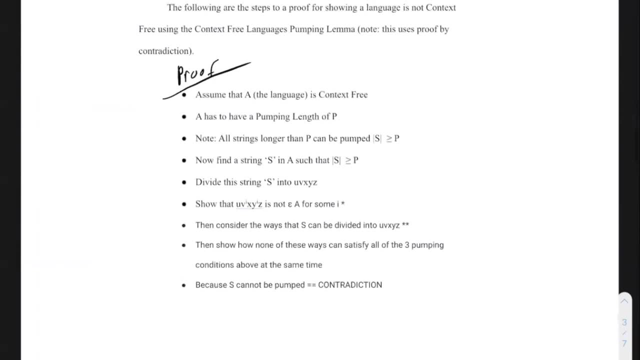 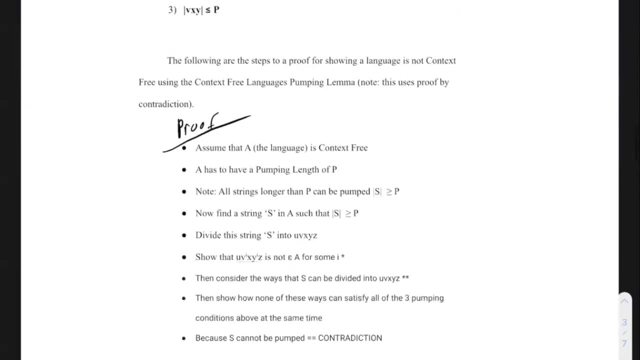 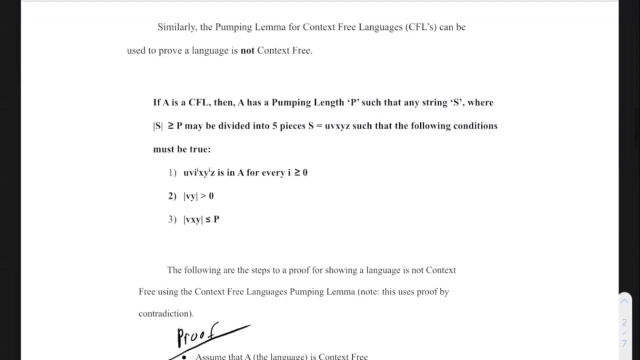 we have these three conditions that need to pass for the pumping lemma And what we do? sorry, I was looking for this part For some power of i. we use it to show that it's not included in the language. And if one, if the example we choose doesn't satisfy, or with one of the cases or both, the 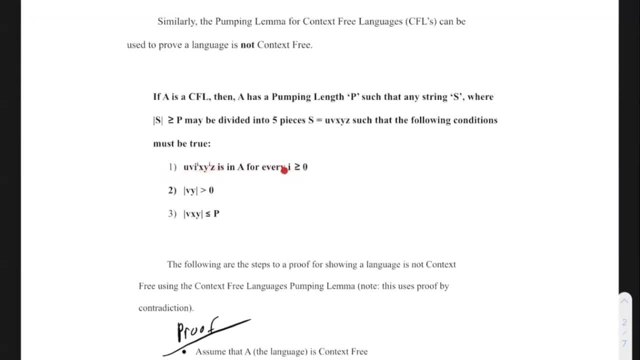 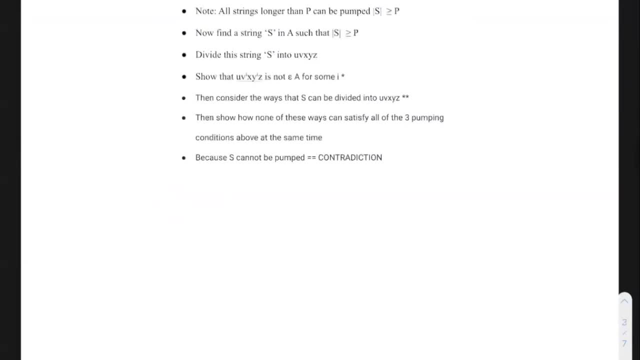 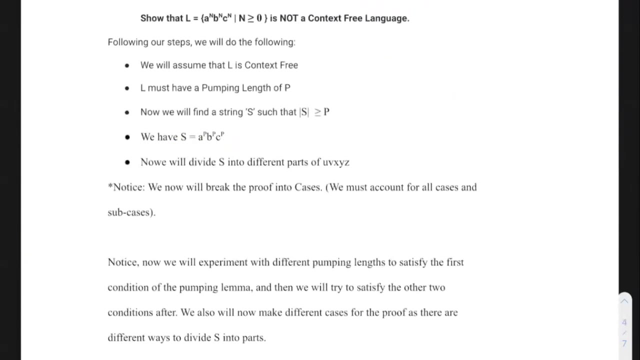 cases. actually, sorry, if it doesn't pass even just one of these, as we did right now, then the pumping lemma does not work with it. So what we did is we followed this basic step until we get to s equals a to the degree of c, and then we choose the powers for degree. 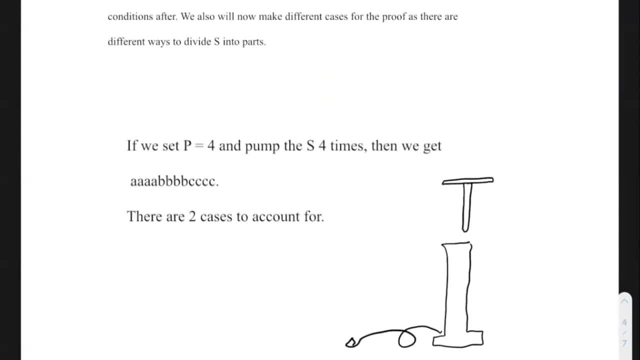 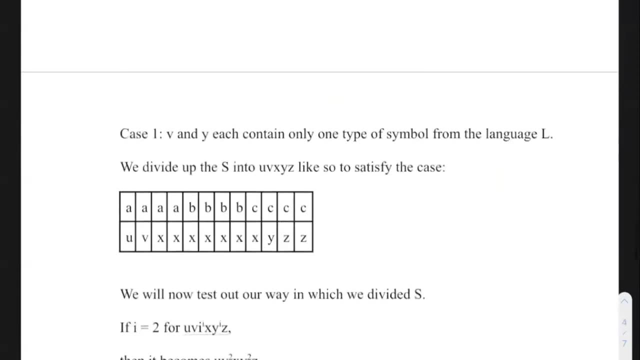 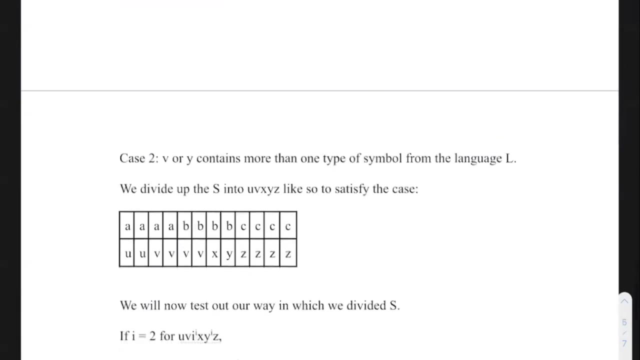 and then we use the same premier method to overcome those and we just put in the number of times that we've presented and we pump, pump, pump, pump it. sorry, I think it's supposed to be four times i It might have been more by accident- And then we got the two different cases where v and y are the 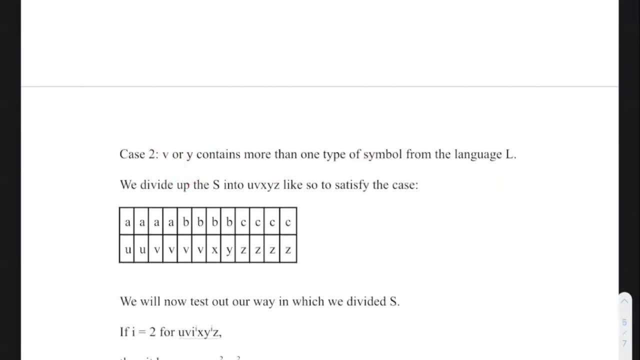 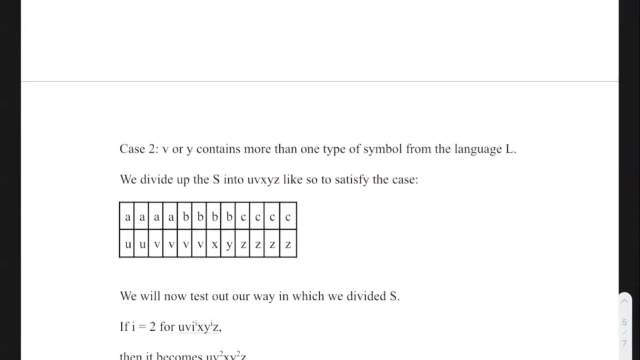 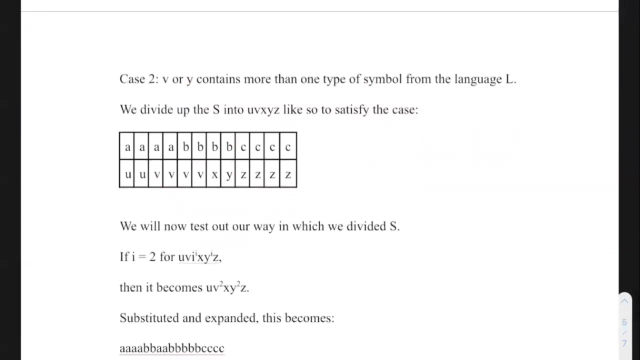 same and they each contain only one type, and also v or y contains more than one type, so they're not the same amount and one of them contains this case for y. it contains only one b, And in both these cases, in the first place, 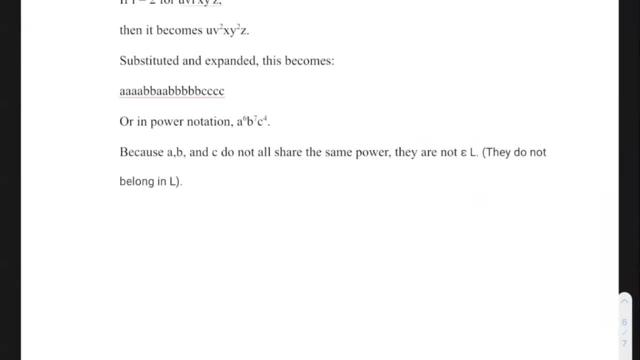 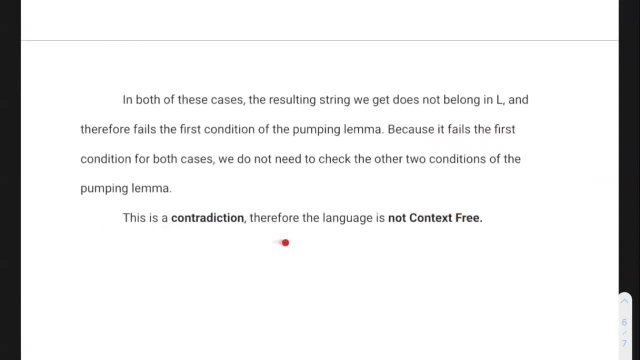 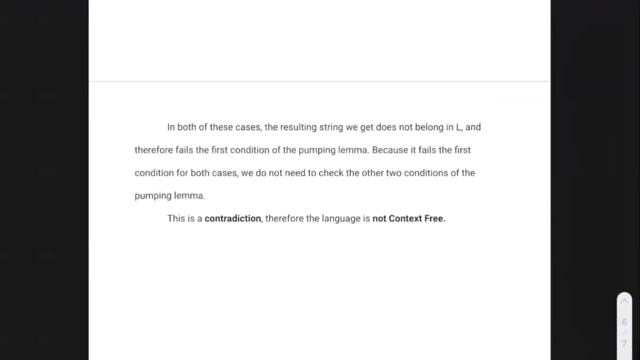 they aren't in the L, So it doesn't satisfy first condition And therefore we have a contradiction. Sorry, And the language is not context-free, And that is everything. Awesome, Thank you.